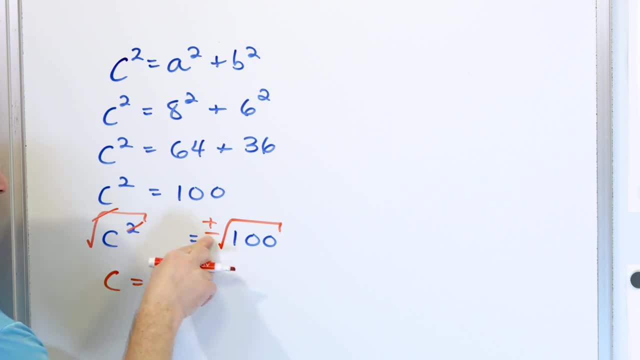 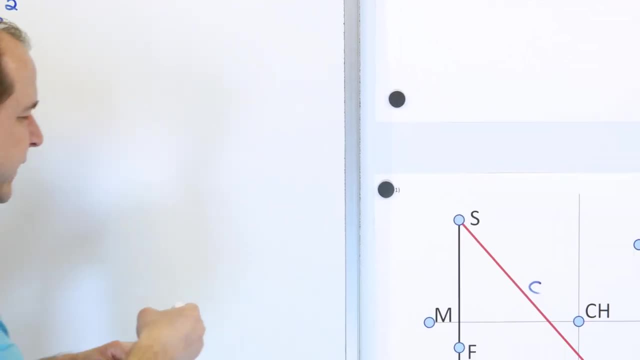 And then what we have is the square root of 100, which is 10.. We're going to throw away the negative because we don't have negative distances. So 10, what 10? kilometers? So if we were to construct a grid system on a map where city hall was in the center and everything was measured relative to it? 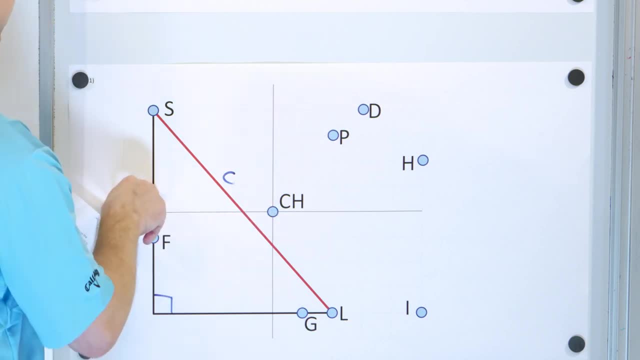 right And you would go. you know this many distance units to the left and this many distance units up to get to the school and similar thing down to the library. then the straight line distance between them would actually be 10 kilometers, as we've shown mathematically here. Let's take this one down and solve our next. 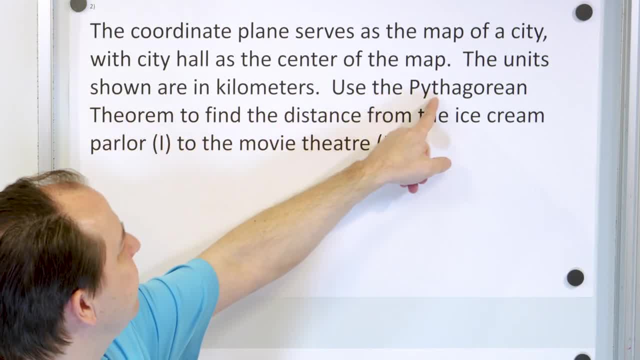 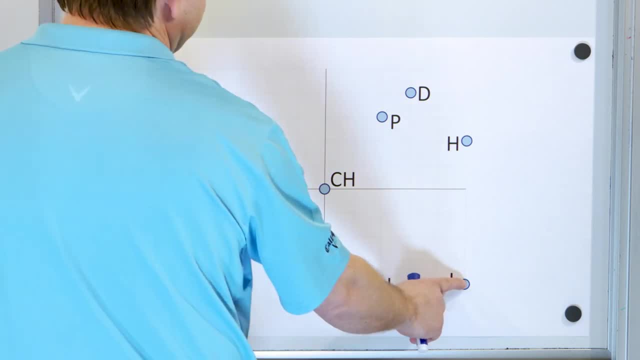 problem. All right, let's take a look at problem number two. We're going to use the Pythagorean theorem to find the distance from the ice cream parlor I to the movie theater M. So the ice cream parlor is here and the movie theater is here. So we're trying to find this straight line distance. 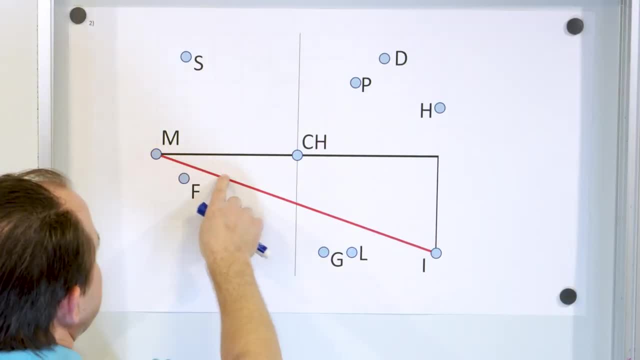 So let's draw that distance and a triangle that fits. Here's the straight line distance. Now we could draw a triangle down here, But it's fine to draw a triangle like this. Either way it's going to work because the distance here. 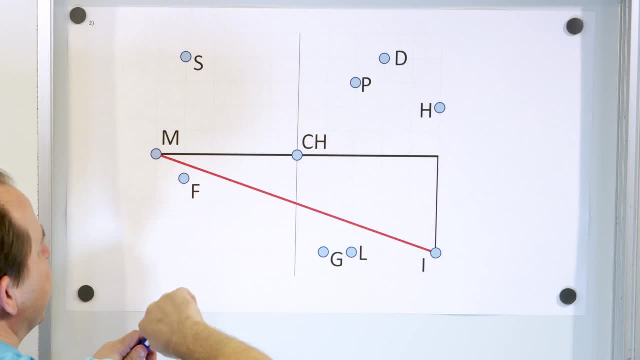 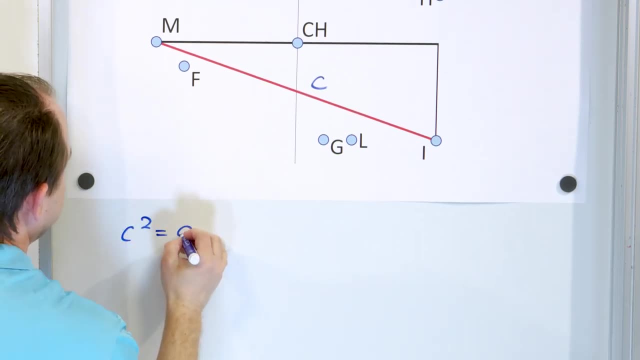 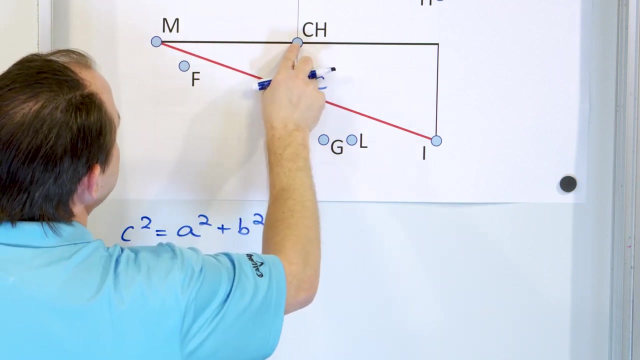 is the same as the distance here, and the distance here is the same as the distance here. So you're going to get the same answer. The hypotenuse C is what we're trying to find here. So C squared is equal to a squared plus b squared. Now C squared is then equal to one side. here is 12345678910.. So 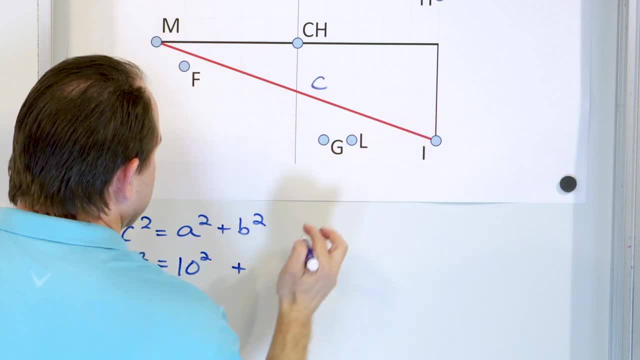 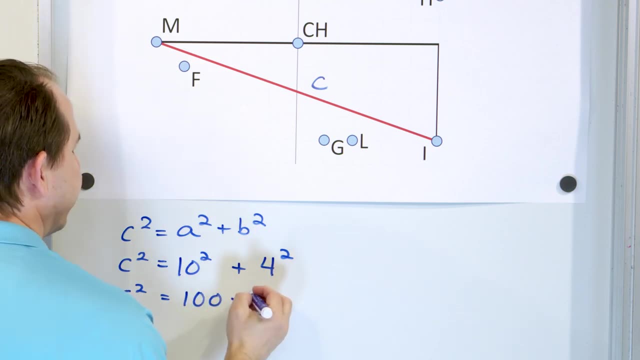 let's go Now the other side. here is one, two, three, four, four squared, So we have 10, squared is 100.. And then four, squared four times four is 16.. So we have C. squared is equal to the whoops. let 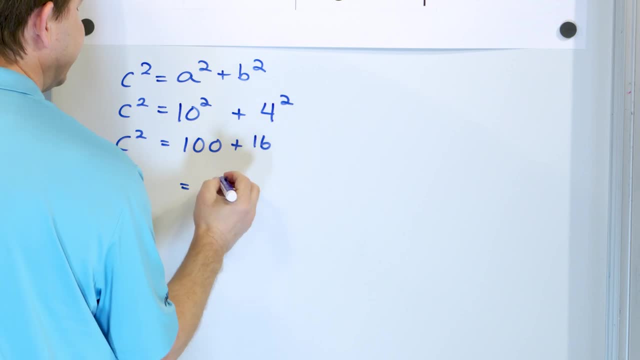 me get too far ahead of myself- is 100 plus 16116.. And in order to solve for that, we're going to do the opposite of the square. we're going to apply the square root and add our plus or minus here, And so we have the distance. C is equal to the dy by c. So then we're going to, we're going to call this: 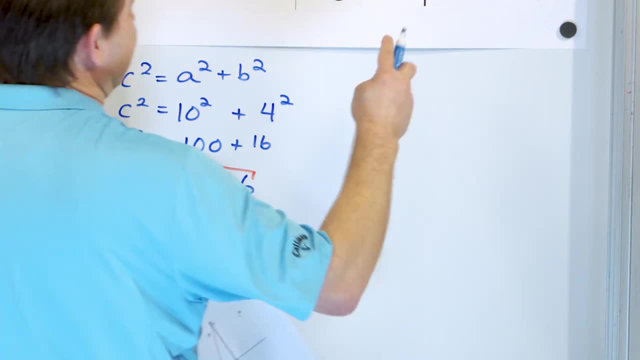 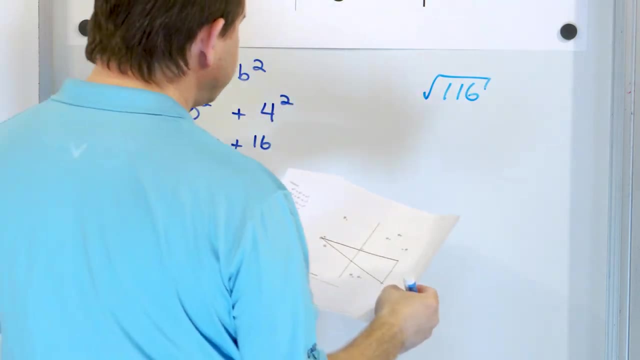 this. So we have to figure out what the square root of 116 is. So we go over here and say: what is the square root of 116?? Now you know, it's an even number, so it's divisible by 2, but it turns. 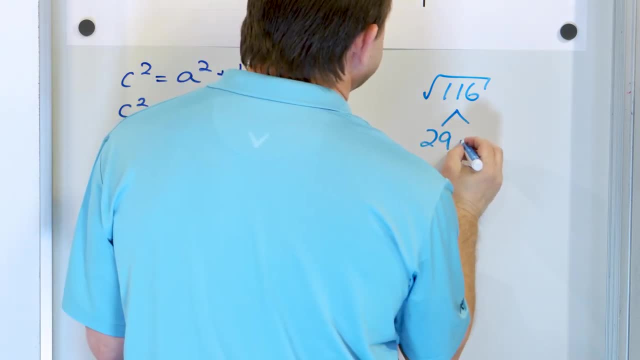 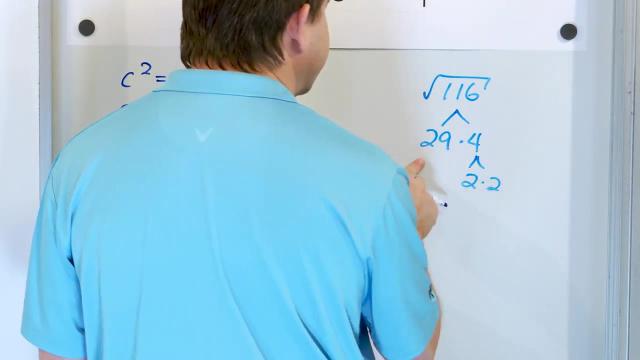 out that it's also divisible by 4.. It turns out that 29 times 4 is exactly equal to 116.. Now this is 2 times 2, and this is not really able to be broken up into anything that's going to have. 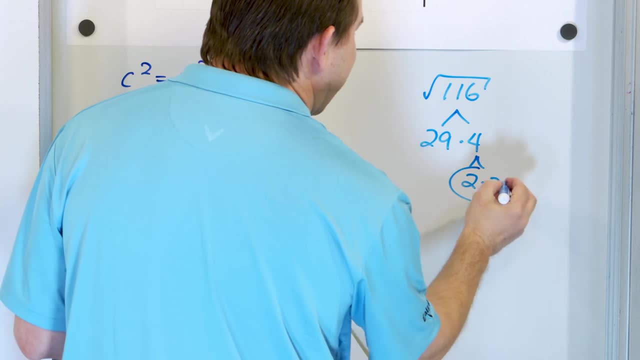 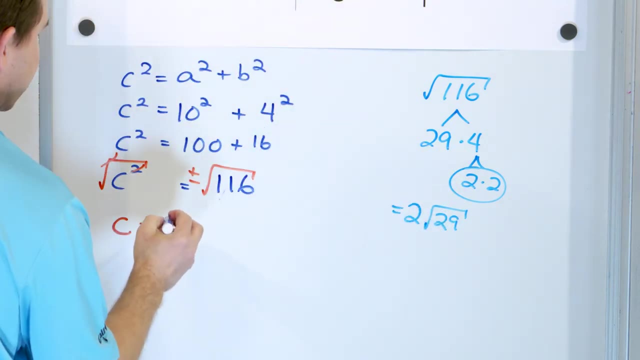 pairs, so you just leave that there. So what you end up with is a pair of 2s which comes out as 2 times the square root of 29.. So the 2 comes out. this stays under the radical, so it's 2 times. 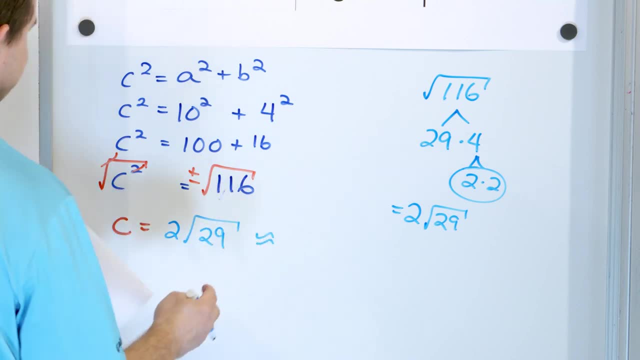 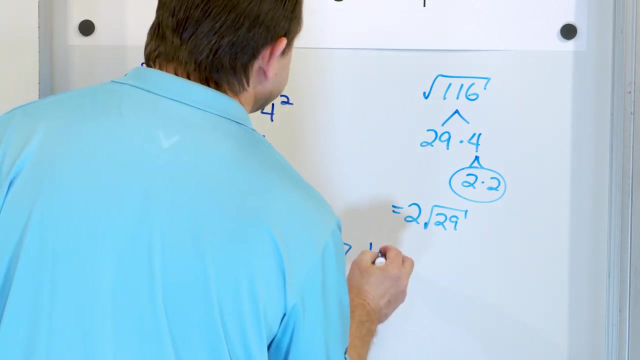 the square root of 29, which is approximately equal to 10.77, and it's rounded, of course. So 29, square root of 29 times 2 is this, and also square root of 16 is this: These are the same thing. so this is the final answer, and the unit here is in kilometers. All right, so just a little. 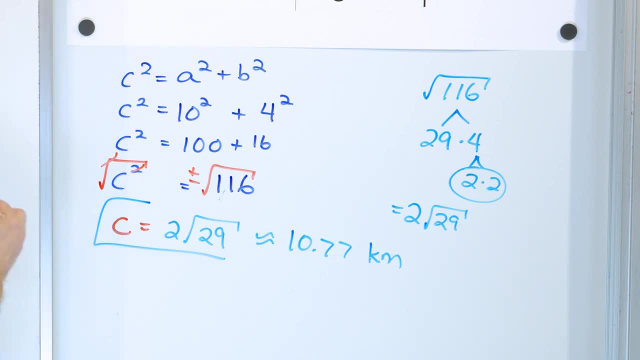 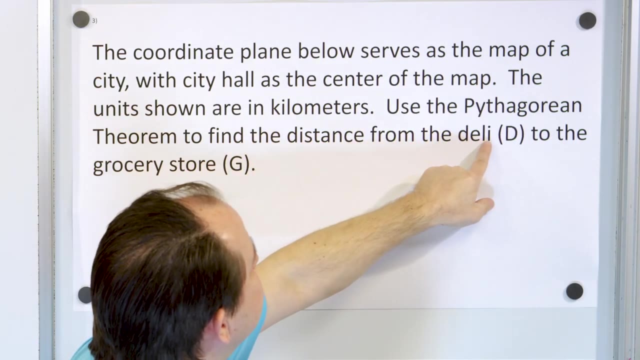 bit over 10 kilometers, close to 11 kilometers. is that distance? All right, we'll take this one down and do our last problem. And here is our last problem. We're trying to find the distance between the deli d and the grocery store g Deli to the. where is it? 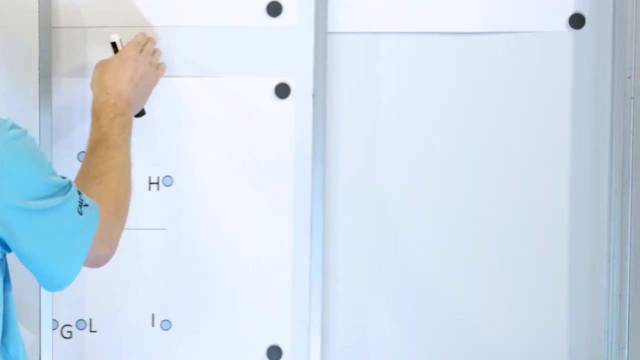 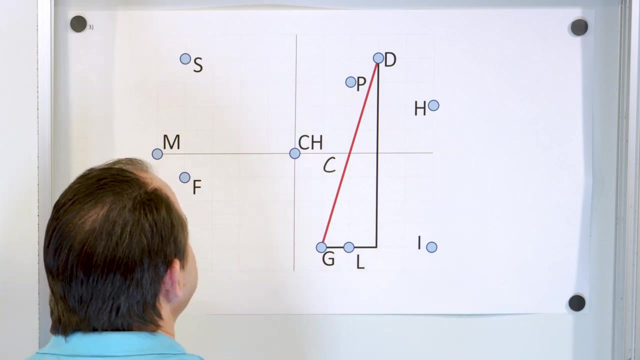 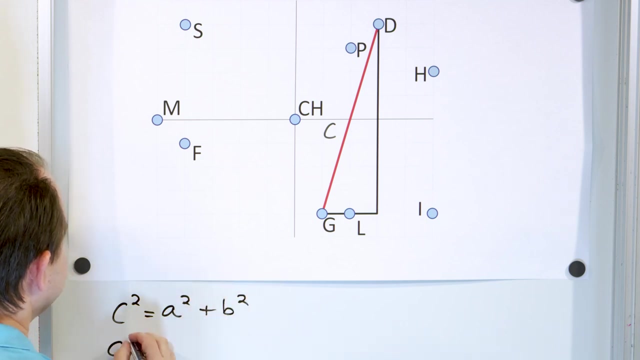 grocery store. So this straight line distance, let's draw that distance here, It's from the deli to the grocery store. We can form a right triangle, of course, right here, and so the red line is the hypotenuse c. All right, so c squared is a squared plus b squared. So we're trying to find. 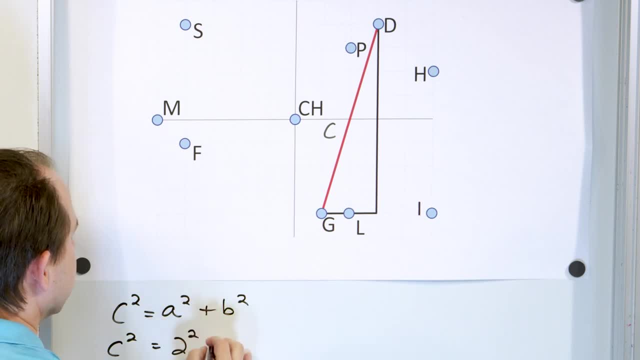 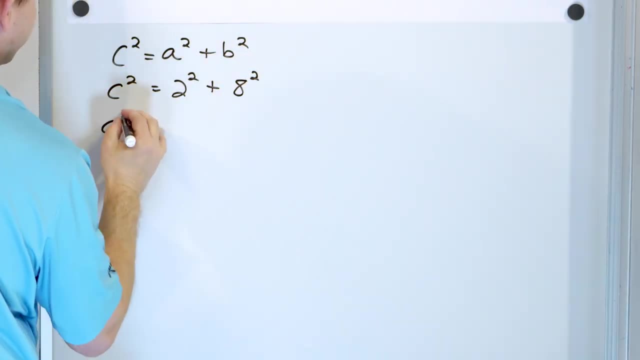 c. I have two distance units here, so 2 squared. and then we have 1, 2, 3, 4, 5, 6, 7, 8 in the other direction. So we have 8 squared up here. and so 2 times 2 is 4 and 8 times 8 is 64. So c squared is: 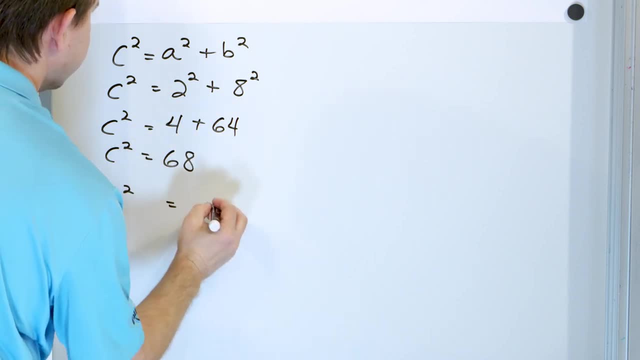 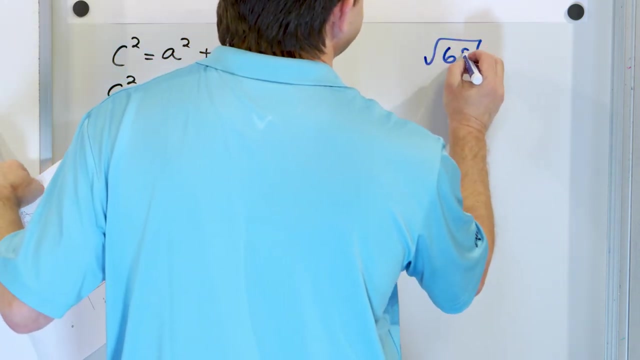 this becomes 68. So c squared is 68. Now we want to solve for c the distance c here. So we're going to take the square root of both sides, cancel these guys, We have to add our plus or minus and the distance c is going to be the square root of 68.. I don't know what that is. So what times? what is? 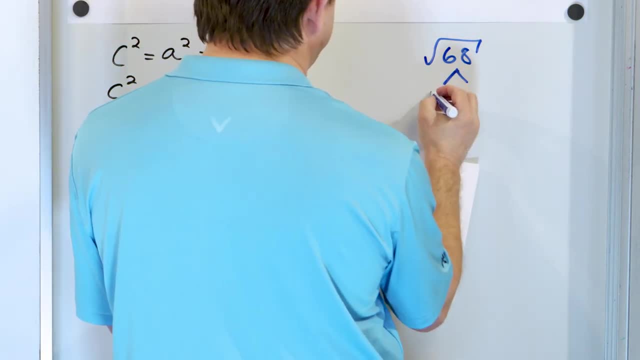 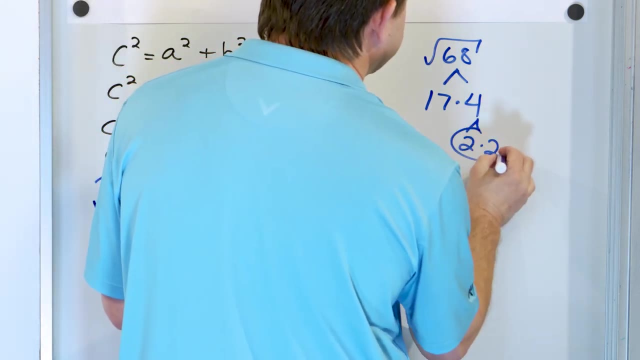 68?? Well, it appears that it's divisible by 2, but it turns out this is divisible by 4 as well. 17 times 4 works out to be 68. And then the 4 is 2 times 2.. I'm looking for pairs, So the 2 comes out.